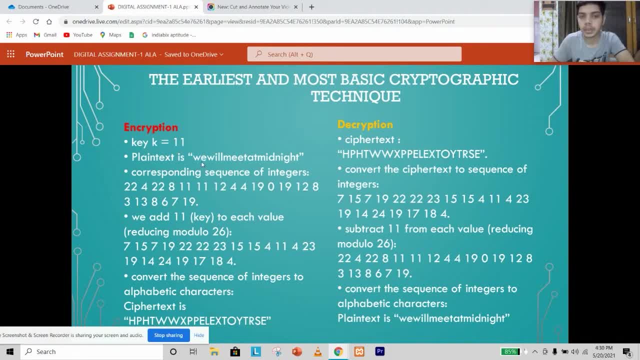 is ır, one taken as 11.. So what we'll be doing at first, we'll be converting this plain text into its numerical equivalents. For example, the numerical equivalent for w is taken as 22,, for e, it is taken as 4, and so on. Now, what we'll be doing for encryption purposes is that we'll be adding the 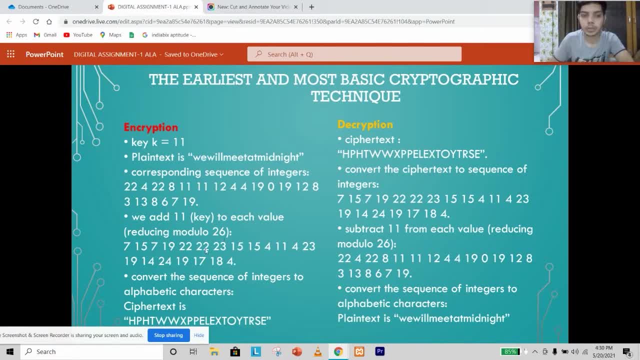 value k using the reducing modulo 26 operator, and we'll be converting this into this particular sequence and again, we'll be converting this into the alphabets back again. So we'll be getting this text, which is our cipher text, Now for decrypting purposes of using this cryptographic technique. 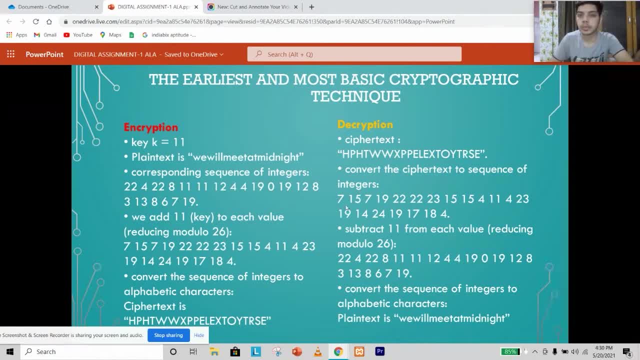 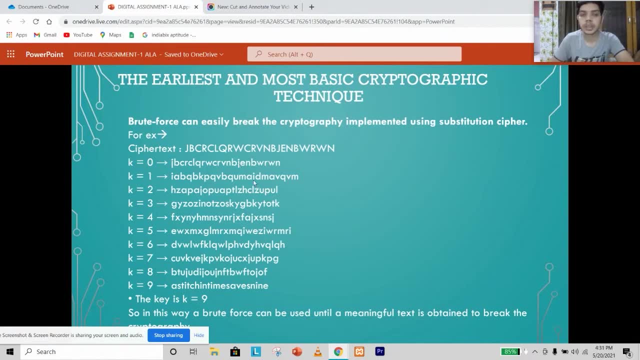 we'll be subtracting the same key from the numerical values that we get. So, as you can see, this particular cryptographic technique is very weak and it can easily be broken down by hackers Using brute force technique. this method can easily be broken down by the hackers who want to. 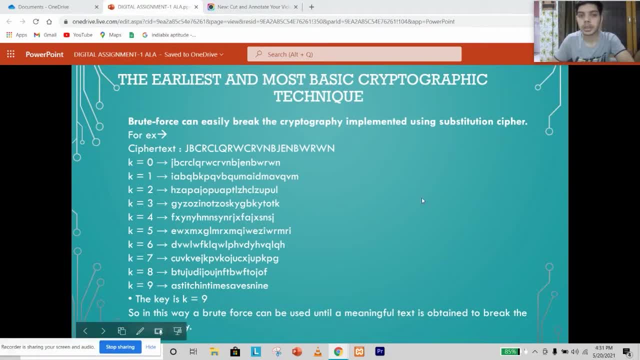 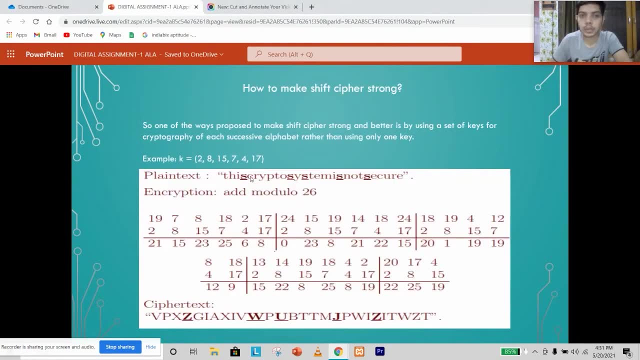 steal our information, So we need to adapt or go to a higher level of cryptography. and for that purposes, what do we do is that, if you want to make the substitution cipher strong, what do we do? That we take a set of keys instead of just a single key and we add this set of keys with the numerical values of our alphabets. 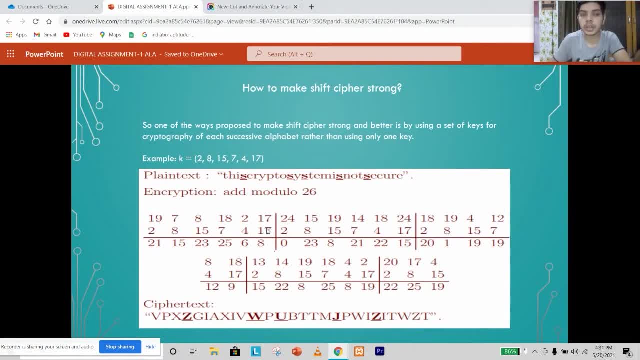 So by doing this we increase the security by a large amount, But still, if we, if the hacker wants to access the information, he can easily do it by using the brute force technique on various keys possible. So we'll be taking the cryptography to a completely new level with the introduction of linear. 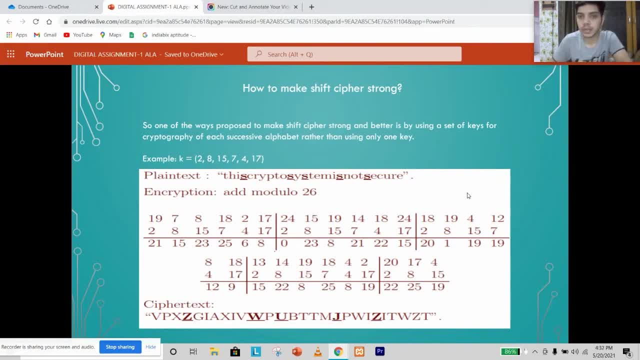 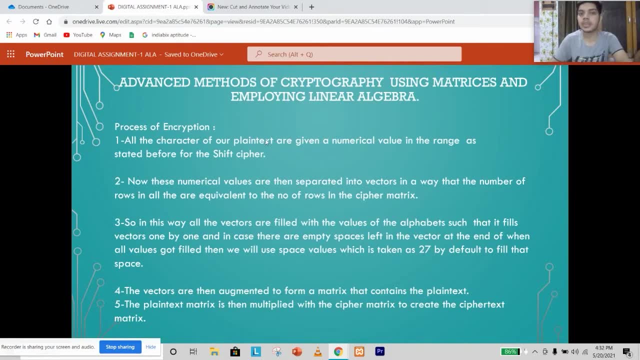 algebra and matrices as keys, which we- which I'll be covering in the next session. So here is the theory related to how do we use matrices for the purpose of encryption. So let us cover all the points one by one. So what do we use? 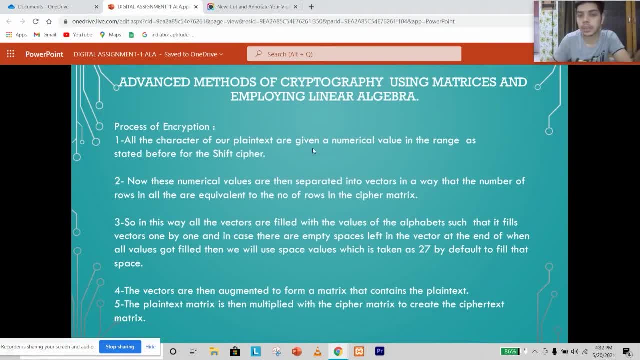 We do first is that we again convert all the plaintext alphabets to the numerical values. Then what do we do is that the values are separated into vectors. the values that we'll be getting will be separating them by vectors and will be arranged in a, in a matrix form. 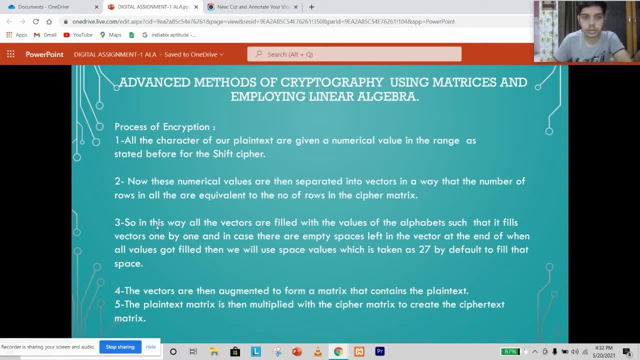 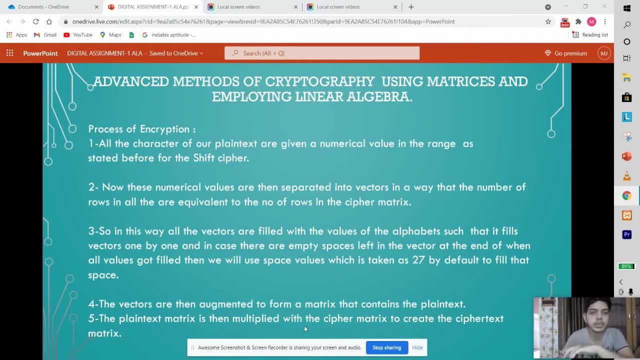 The next step that we do is that: OK, OK, guys, so now we'll be seeing the complete process of encryption and decryption using matrices and the linear applied applied linear algebra. So this is a complete process of encryption over here, So you can basically give it a read. 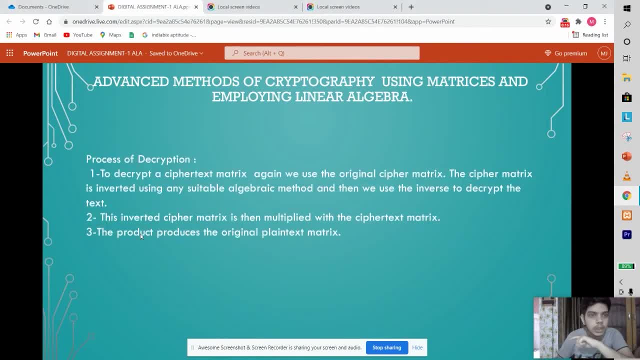 I'll be explaining each and every point with the help of a suitable example. Similarly, this is a complete process of decryption. You can again give it a read. I'll be explaining all the points thoroughly with the help of a suitable example. So, before jumping directly into the example, I'd like all of you to just remember this particular table. 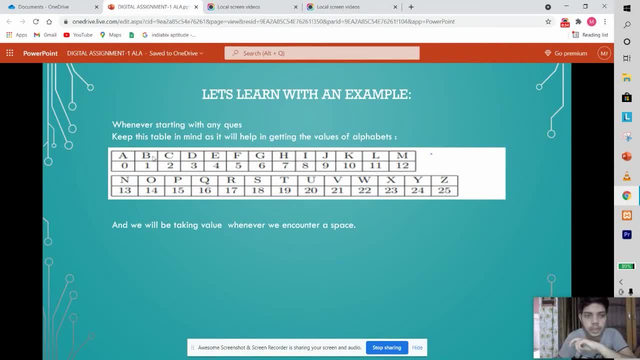 This table is used for the purpose of converting the alphabets of the plaintext That we will be getting into the numerical equivalents. for example, a numerical equivalent is zero, B has a numerical equivalent as one, and so on. Similarly, for if we'll be encountering a space in between our particular plaintext, then we'll be using the numerical equivalent of 26.. 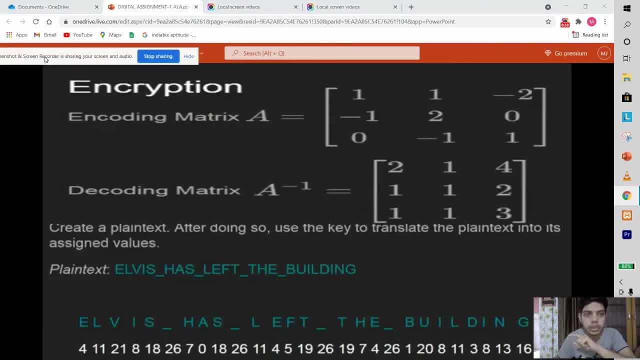 OK, so now let's jump into the example. So this is our very first example. The plaintext that we have over here is: Elvis has left the building and this is our encoding matrix. So the very first thing that I want all of you to realize is that the encoding matrix in this particular case is same as the value of K in case of the substitution cipher. 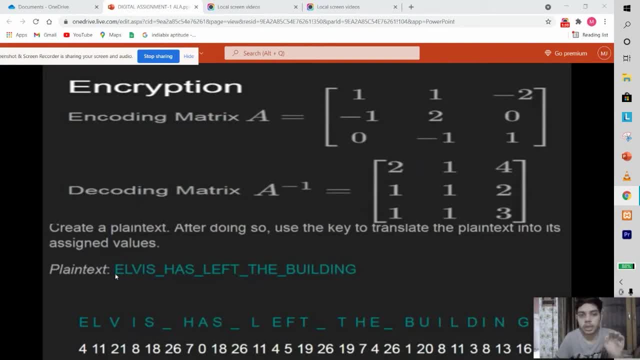 We'll be using this encoding matrix for the sole purpose of converting our plaintext into ciphertext. OK, so now let's jump into the process of encryption. So the very first step that you need to do is that you need to convert this plaintext into the numerical equivalent. 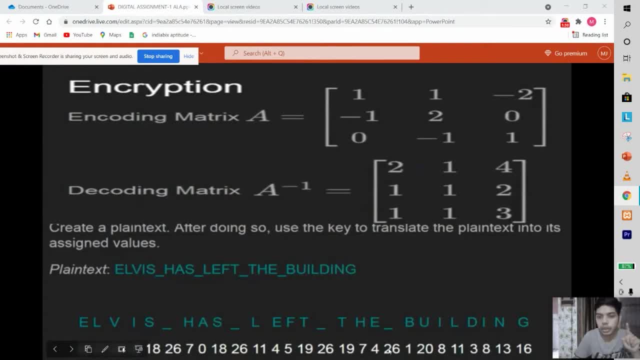 The sequence Of numerical equivalent values. as I've shown over here, we'll be using the same table that I've shown you for this purpose. We'll be converting the plaintext into a numerical equivalent. So this is our first step. Now the second step: we will be making vectors of row size three from the sequence that we have just obtained. 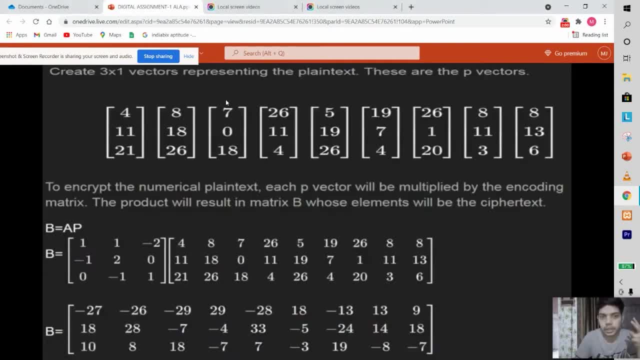 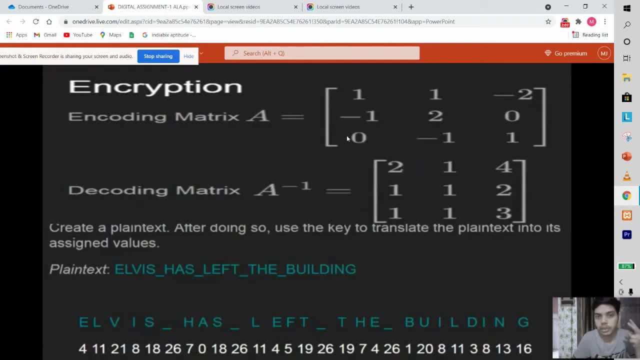 As you can see over here, we have made vectors of row size three from the sequence that we have obtained earlier: 4,, 11,, 21.. So the reason for row size three is that the row size need to be same as the row size of the encoding matrix. 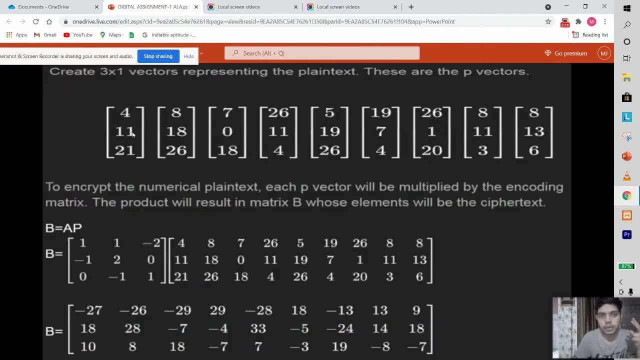 So over here we have the row sizes three, So we will be forming vectors of row size three over here also. Now the third step is we'll be combining all these vectors and we will be multiplying it with the help of the encoding matrix. 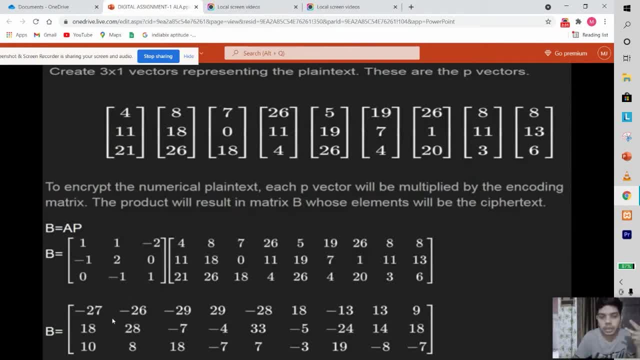 So this is basically a basic matrix multiplication. The answer to this multiplication is shown over here. Now the fourth step is we will be again separating the vectors of this matrix. just like we have done over here, We'll be separating the vectors of this particular matrix. 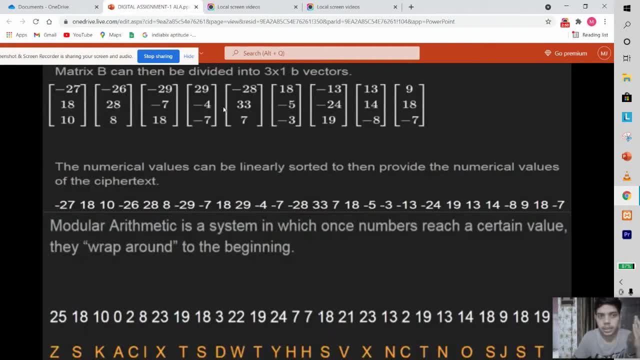 Let me show you how, in this manner, we will be separating the vectors of this matrix. So now the fifth step. what we will do is that we'll be arrange all the numerical values of this vector again into a sequence. Now this particular sequence: 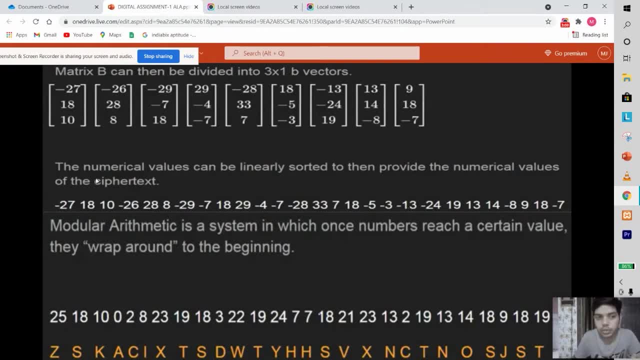 It represents our ciphertext but, as you can see, minus 27 has no place in the table where I was converting numerical values into alphabets. So to get this, for these values, the negative values, as well as the values which are greater than 26,- we will be applying the modular arithmetic operator. 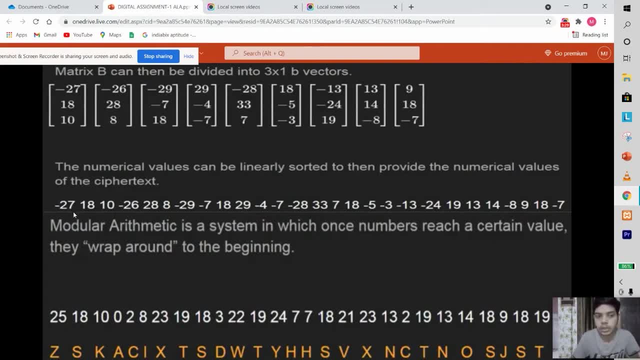 We'll be basically taking the mode of all these values with 26.. So the resultant sequence will be like this, And this over here is When we will convert this particular numerical values into alphabets, using the table that I have shown you earlier. 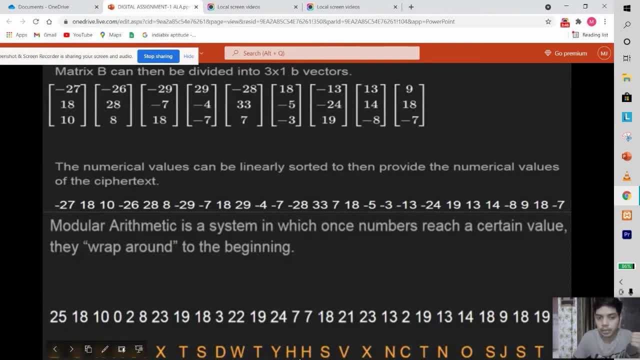 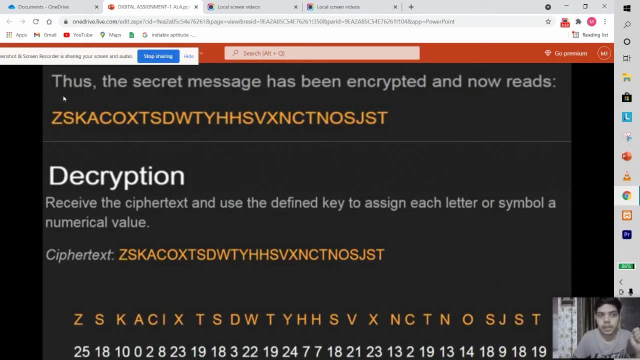 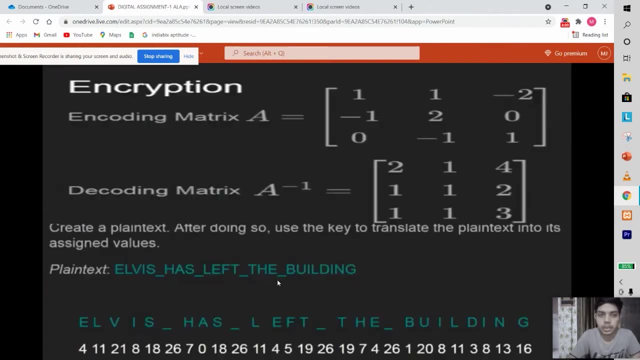 This, particularly this particular alphabet sequence, is our ciphertext. So this is a complete process of encryption. We have converted our in text that is always has left the building into a ciphertext. So let me just revise the complete process again. Firstly, we'll be 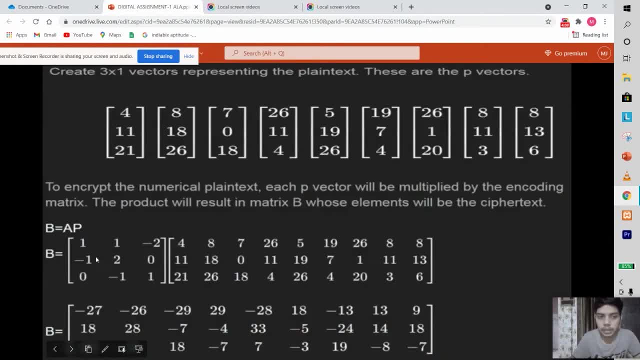 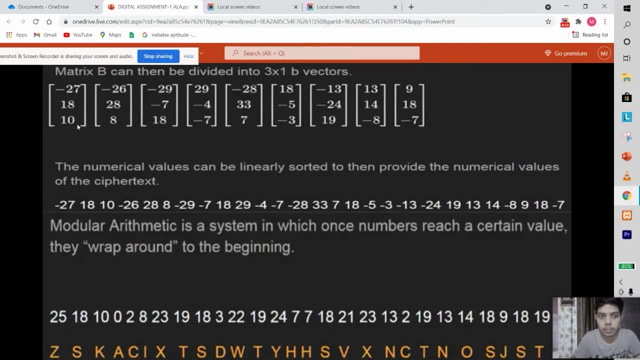 Forming the sequence. Next, we will be multiplying the vectors obtained by the encoding metrics. The next thing we'll be doing is we'll be arranging the multiplied metrics back into a sequence of numerical values. We'll be applying modular arithmetic and we'll be getting the ciphertext as here: 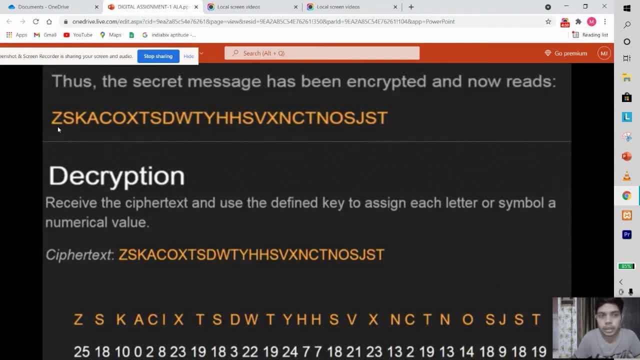 OK, so this is a complete process of encoding encryption. Now we'll be moving to the process of decryption. So the process Of decryption is very much similar to the process of encryption. We'll be following the exact same sequence of steps as we have followed in case of encryption. 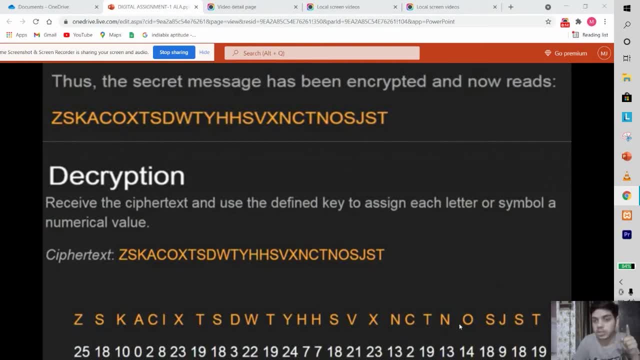 So the very first step that we followed in encryption was converting the sequence of alphabets into the numerical equivalents. So this is our ciphertext. We'll be converting the ciphertext into the numerical equivalents. So this is our first step. The second step that we followed in encryption was to arrange this sequence. 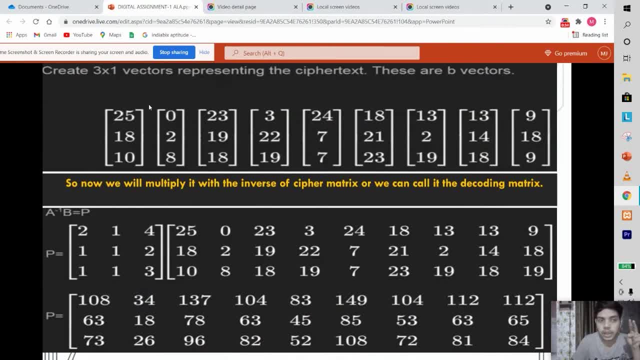 In To vectors of row size three. So the same process I have done over here, I've converted the sequence into vectors of row size three. The third step in the process of encryption was multiplying these sequence with the encoding metrics. But over here, as we are decoding the ciphertext back into the plaintext, we will be multiplying it with the inverse of encoding metrics. 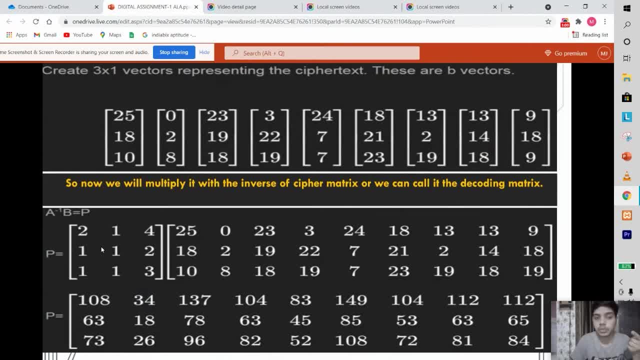 So for the purpose of getting inverse, You can use various alphabets, various linear algebra, algebraic methods. For example, you can use Gauss Jordan method for obtaining this inverse. So once you have obtained the inverse, you will be multiplying it with the sequence of the vectors that you have obtained. 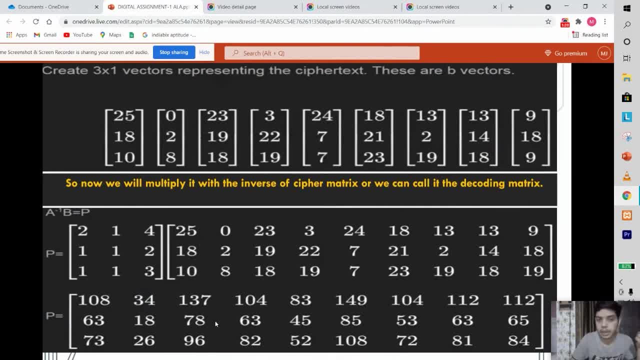 So this is the result Multiplied of the matrices over here. So the again, we'll be following the same steps as we have followed in case of encryption: We'll be separating, Getting the multiplied metrics back into vectors of row size three. 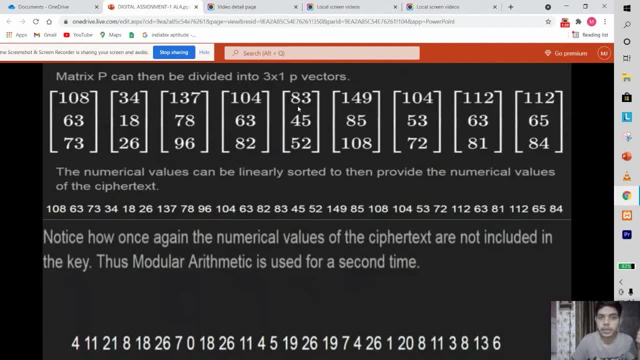 So over here here I have separated it back into vectors of row size three. Again, I'll be arranging all these vectors into sequence: one zero, eight, sixty three, seventy three. one zero eight, sixty three, seventy three, thirty four, eighteen twenty six, thirty four, eighteen twenty six. 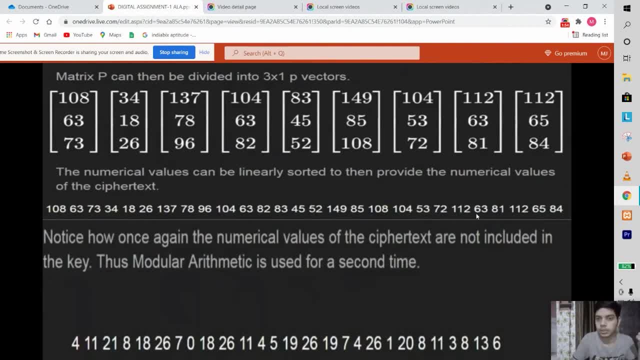 So, like this, I'll be arranging them into sequence of numerical values. So again, as you can see that if I want To convert this back into alphabets, there is no such alphabet for the value one zero eight. So I need to get this value in the range of zero to twenty six so that for that particular purpose I'll be again using the modular arithmetic and I'll be taking the mod of all the values which are greater than twenty six. 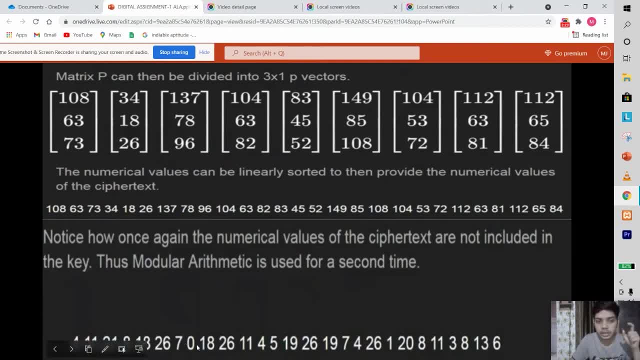 I'll be taking their mod of twenty six, So I'll be getting this particular sequence Now. if you observe this sequence carefully, for eleven, twenty five, One, eight. This is the same sequence that we got when we converted our plain text into the numerical values. 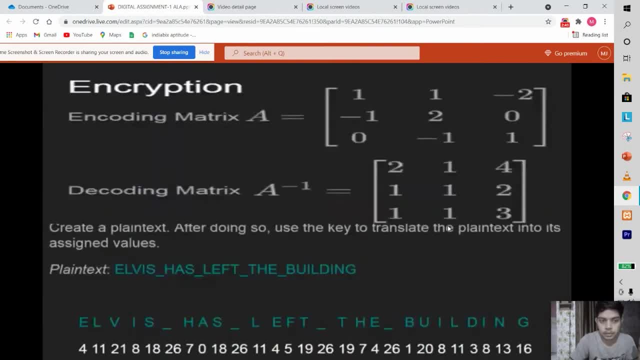 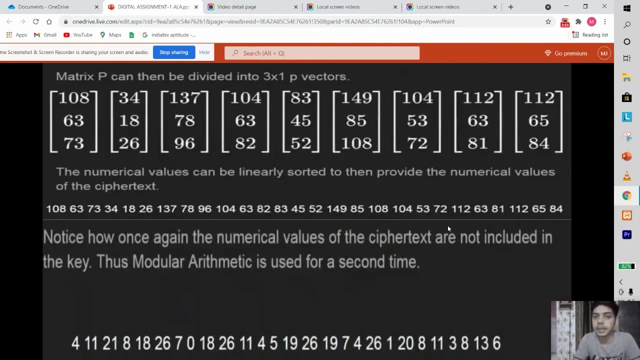 So let me show you This was our plain text. Elvis has left the building and when we converted it into numerical values, we got the same sequence for eleven, twenty one. So even after the process of decryption, we are supposed to get the plane, we are supposed to get back the plain text. 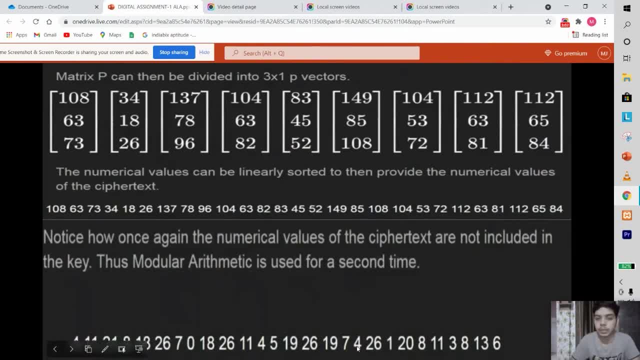 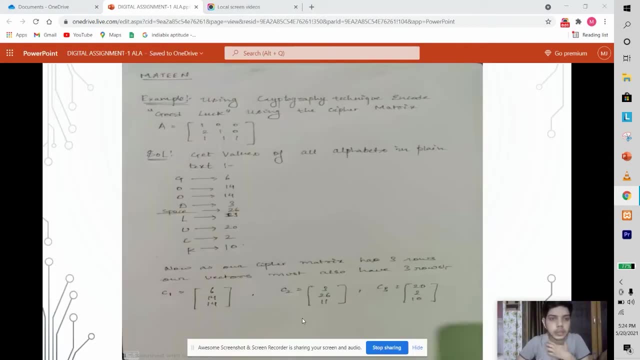 So we're here. We have got the same sequence as we have got from the index, So this basically represent our index. So this completes the process of decryption. So now I'll be taking many more examples for complete understanding of the subject, OK, guys. so for better understanding of taking another example of cryptography over here, 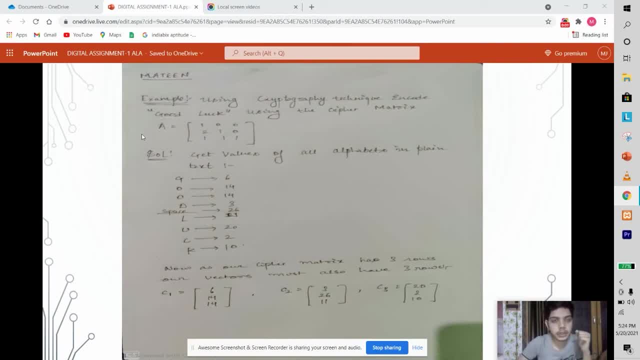 So over here. the plain text that I have is good luck, and the encoding matrix is denoted by a. this is over here. This is our encoding matrix, So we'll be following the exact same procedure, exact same steps as I have followed in the previous example. 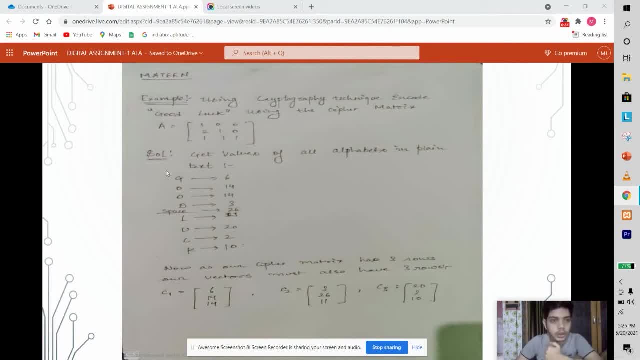 So the very first step was to convert all the alphabets into numerical equivalents. So over here I have converted all the alphabets of my plain text- that is good luck- into the numerical equivalents, OK. so the second step was to organize this, the sequence of numerical equivalents, into vectors of row size equal to the row size. 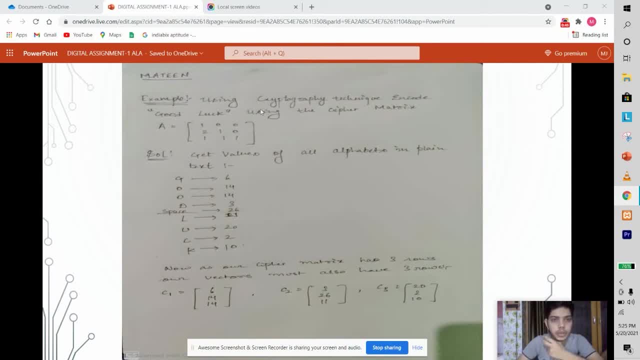 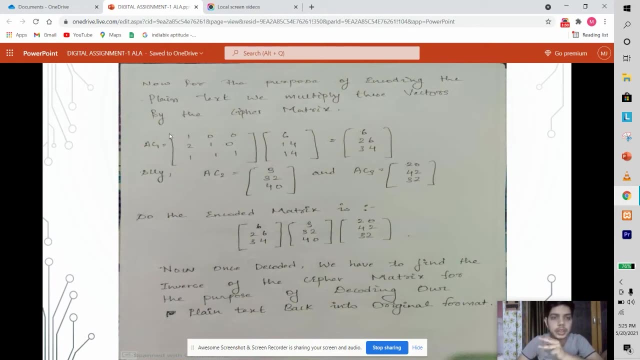 of the encoding matrix. over here We have our encoding matrix, its row size, As you can see, it's the. it's row size is three, So we have arranged it into vectors of row size three. Now the third step was to multiply the vectors obtained with the encoding matrix to get the ciphertext. 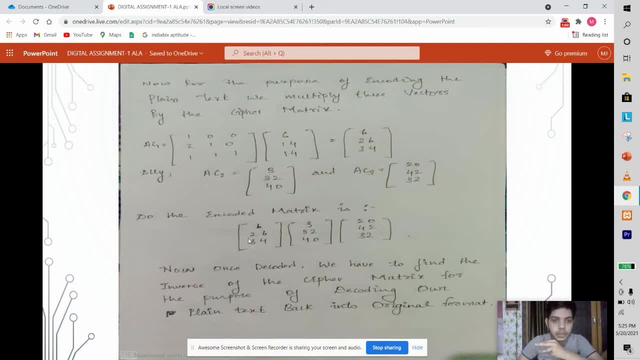 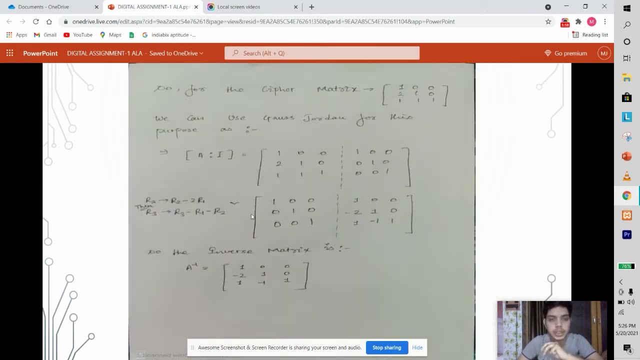 So over here I have shown the multiplication of individual vectors. So this is the this over here is the result of multiplication And this represents our ciphertext. This is the cipher matrix of the ciphertext, as we say. So now the this this was the complete process of encoding. 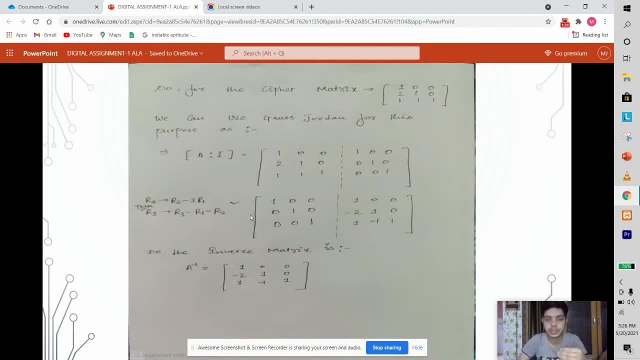 We have taken the plaintext and we have converted the plaintext into the cipher matrix, or the ciphertext as we say. Now for decoding, as I have stated earlier, we will follow the exact same steps, But this time we will be multiplying the matrix with the, with the inverse of the encoding matrix. 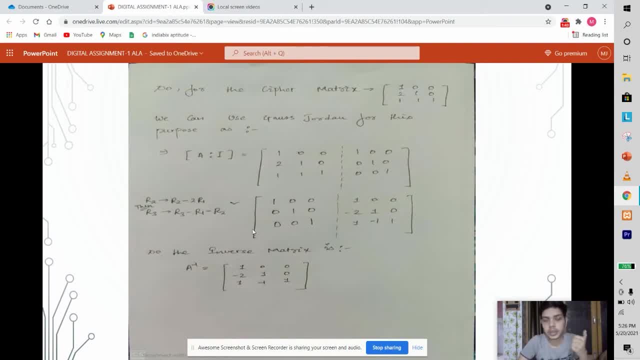 So in the previous example, as I have said that You can find the inverse using linear algebraic methods, for example Gauss-Jordan. So over here I have demonstrated the process of Gauss-Jordan. So basically, what we do in Gauss-Jordan is that we try to convert the given matrix into the final identity matrix using a set of row operations. 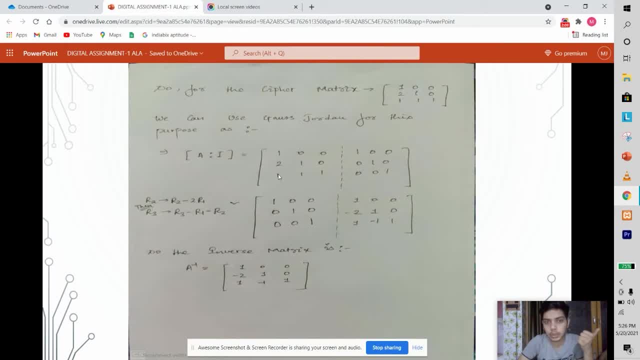 So over here the row operations are stated. You can apply these row operation on this particular matrix and you will be getting, Uh, Identity metrics. So the metrics that we you got alongside the identity metrics after these row operations, represents your, represents the inverse of the metrics that you have started with. 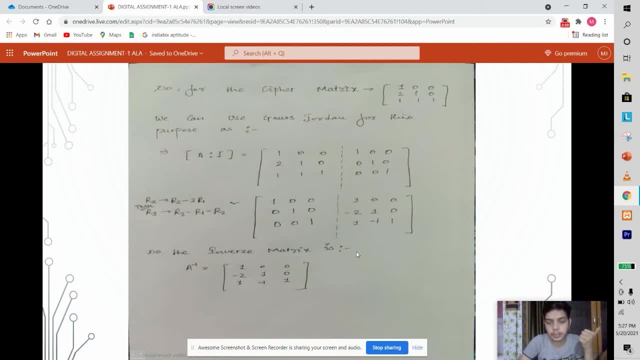 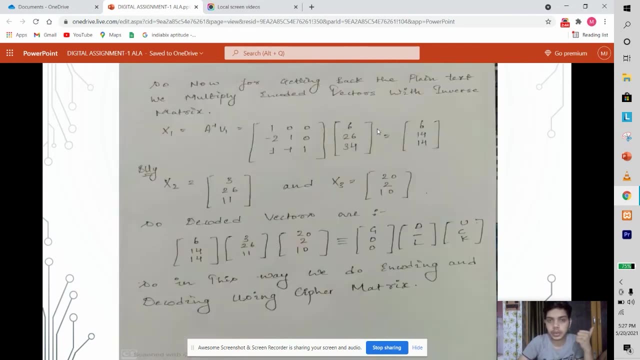 So this is basically the inverse metrics we have with us. We have calculated the inverse metrics using the linear algebraic method of Gauss-Jordan, So now we will be using this inverse metrics for the purpose of decryption. OK, So We have our vectors over here. 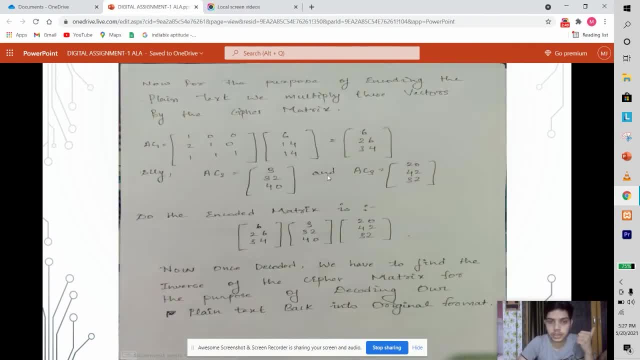 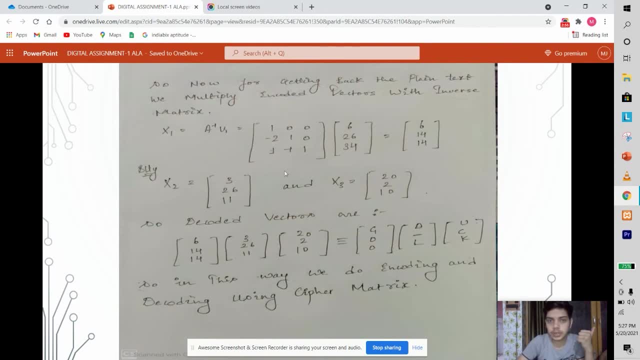 These are the vectors from the ciphertext. You can see these. these are. this is the ciphertext matrix. So we are multiplying the inverse of encoding matrix with the ciphertext matrix and the result that we are getting represents the plaintext. OK, So you can basically multiply all the all the ciphertext vectors with the encoding inverse of encoding metrics. 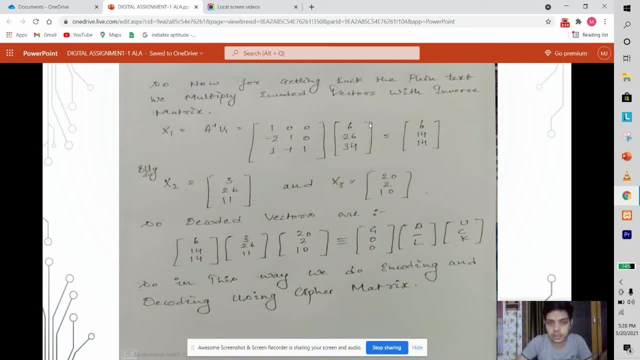 And you will be getting The plaintext vectors. so I have assembled all the vectors over here: 6,14,14,3,26,11,22,10, and if you convert these numerical values back into alphabets, you'll be getting the same plaintext. that is good. space luck. 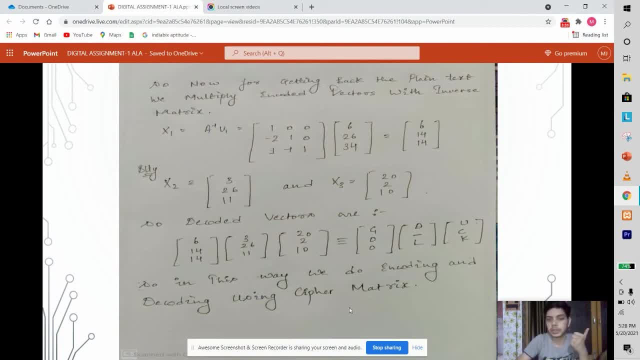 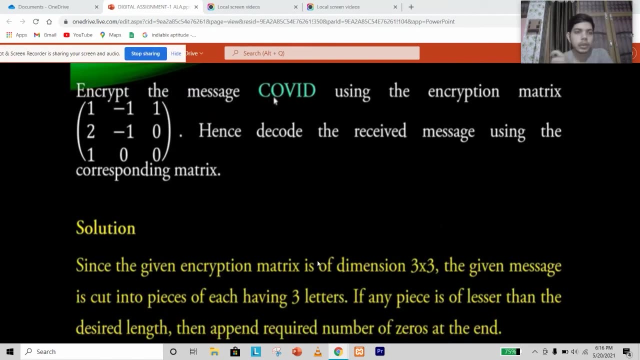 OK, So in. so in this way we do encoding and decoding using cipher matrix or, more precisely, we can say, using linear algebraic methods. So This is all about the examples that I I want to can. OK, So now I just want one last step, one last concept I want all of you to know, and this will be really helpful, especially when you'll be solving a number of problems on cryptography using matrices. 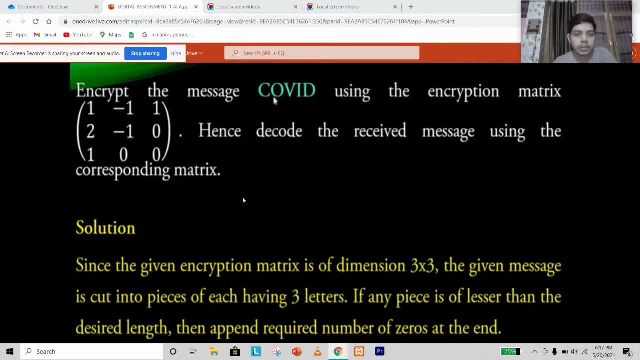 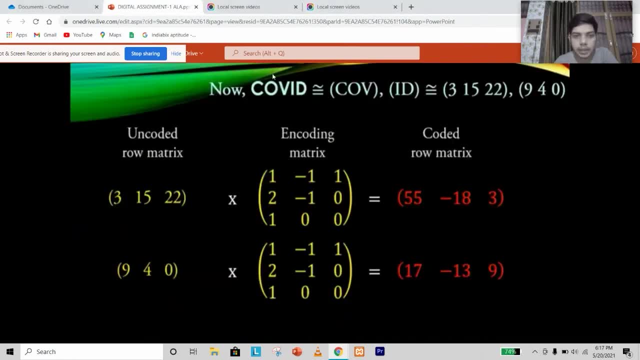 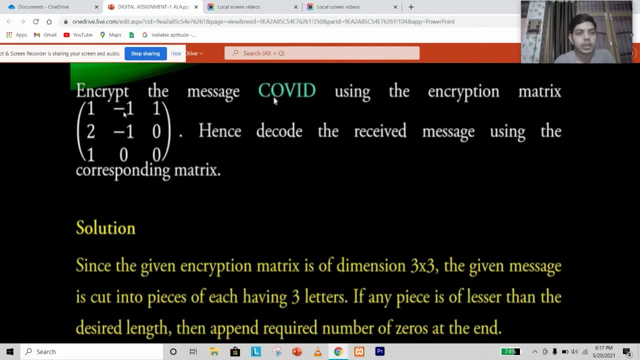 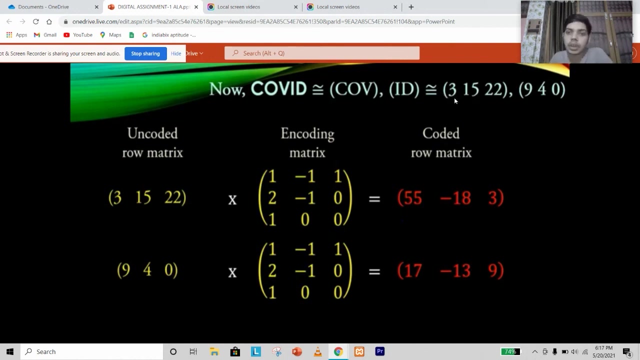 So the concept is that there will be a number of cases when the plaintext that you will have, when you will be converting this plaintext, for example, you have the plaintext as code And because the encoding metrics that you have is a full size 3, you will have to read the sequence and vectors that you will have to generate from the sequence should also be of row size 3, as I've already explained in the previous two examples. 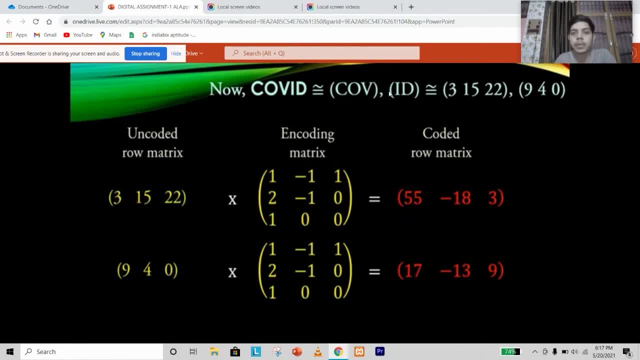 But, as you can see, we only have five alphabets, in this case C, O, V, I D. So we just have five alphabets and we need to form vectors of row size 3.. So The first one, we can easily form using the alphabet C O V, we can form this vector 3, 5, 15, 22. but for the second vector, that is, we are just left with I D, we are just left with two alphabets and we need to form vector of row size 3.. 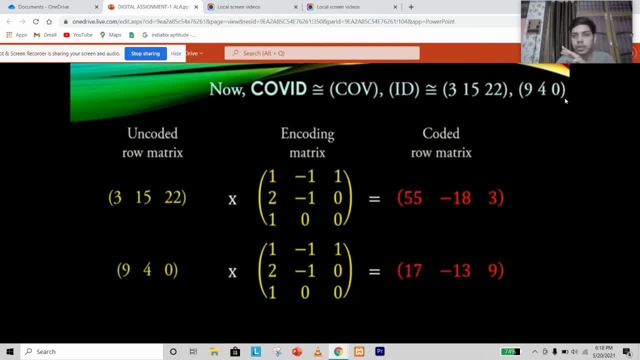 So what do we do in such cases? we add an additional 0 if we are short of alphabets with us. So OK. So for I, we have the numerical value is 9. for D, we have the numerical value is 4.. And 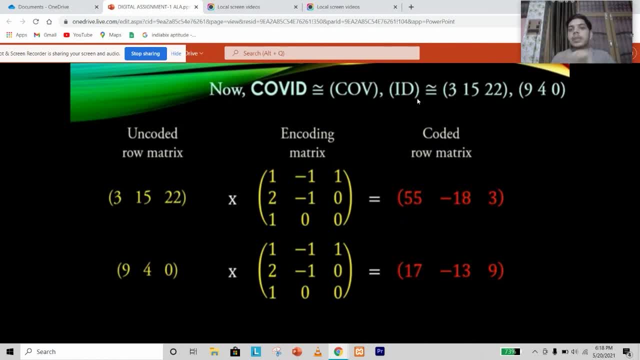 as we have to form vectors of row size 3, so we be adding an additional 0 from our side to complete the row size of the given vector. So the further the process of encoding and decoding is exactly the same. We'll be multiplying this, these vectors, with the encoding vertracless and the resultant vectors that we will be getting will. 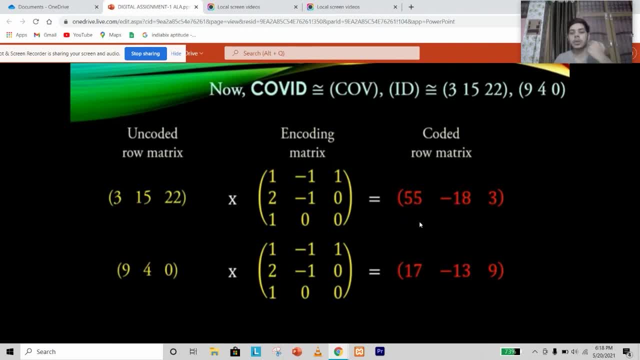 form the ciphertext. So this is all that you need to know for the purpose of using Vectors, Vectors, Vectors I, And also Vectors after that, Por applying or writing, And so cryptography using linear algebra and matrices. so, finally, i would like to highlight the references: